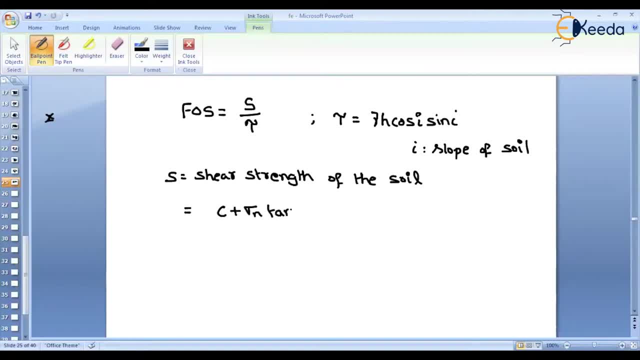 plus sigma n into tan phi s. So in this equation, h is nothing but a shear strength and che is nothing but a cohesion of the soil and pragmatism, and sigma n is nothing but a normal stress acting on the plane 22.. 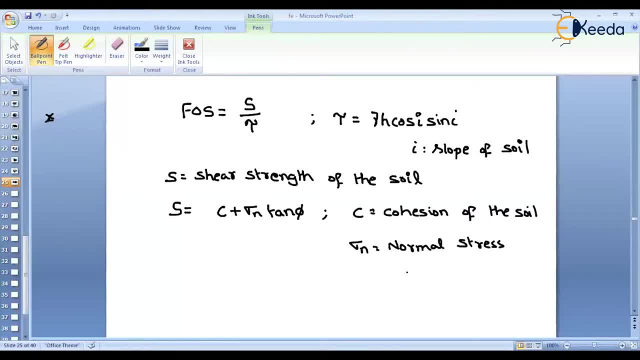 3. 14. 17. normal stress acting on the plane considered, and phi is nothing but a angle of friction. okay, so by using this c plus sigma and tan phi, we can find out the shear strength of the soil at any layer and at that layer we can find out what is the shear stress acting on the 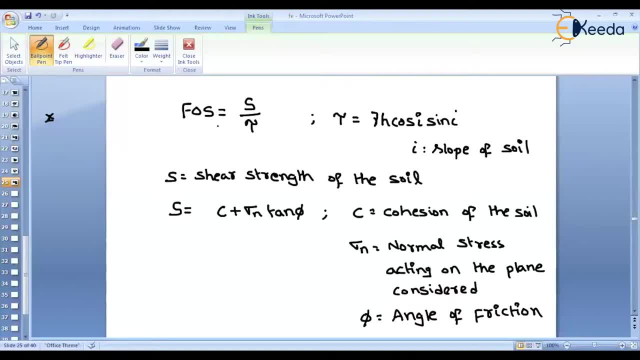 layer. so, depending by using this equation, we can find out the factor of safety. if it is comes greater than one, we can say the soil mass is stable at that layer. if it is coming less than one, then we can say that the soil will be failure. okay, now let us consider that. 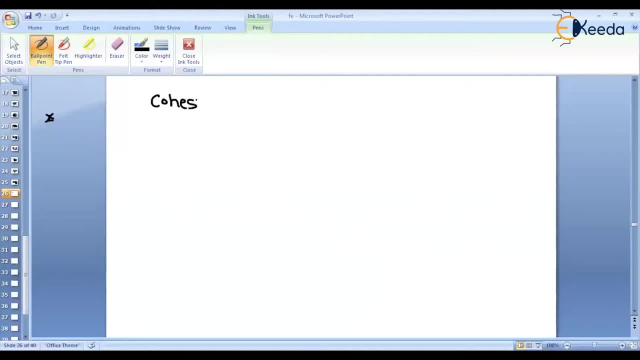 in this video we are discussing about only cohesion with lessذا. so what is mean by cohesion with lessza? what are the examples? either these are maybe gravel soils, or else sandy soils, so otherwise we can say that coarse grain soils. what are the examples? gravel, sand and all. 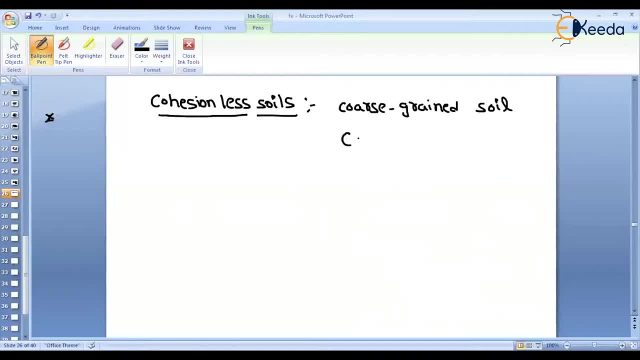 what is mean by gosp creation less the term emblems cohesion. that means c value will be equal to zero. so if c equal to zero, what about your shear strength equation? your shear strength equation is becoming the sigma n tan phi. That means wherever you are finding. 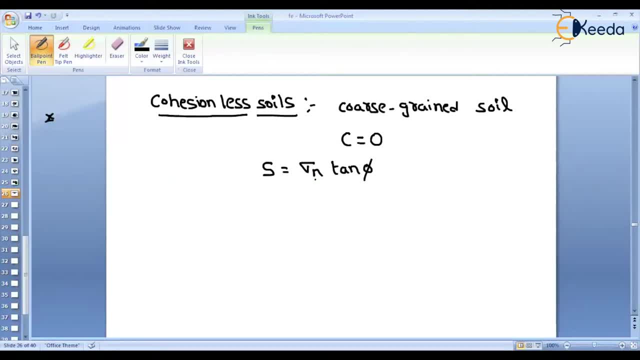 the shear strength at that layer. sigma n is nothing but a normal stress acting on that layer. By using the angle of friction we can find out the shear strength of the cohesionless soils. So first let us consider that we are considering the dry soil. So if we are considering 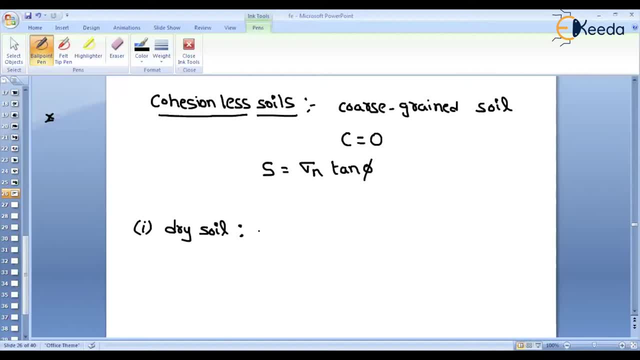 the dry soil. so you have to consider dry density of the soil while doing the calculation part. So that means there is a gamma will be equal to. if it is a dry soil, then we have to take gamma will be equal to unit weight of the soil. 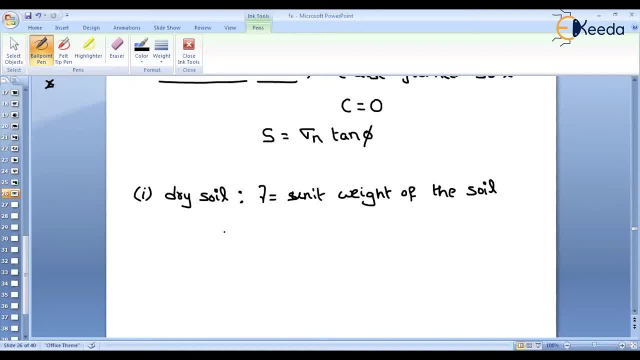 So how your equation will be coming. So your shear stress on the failure plane that will be equal to gamma, into h, into cos i, sin i, and shear strength at that plane will be equal to sigma n, Sigma n, if I replace with gamma h cos of square i and also tan phi remains. 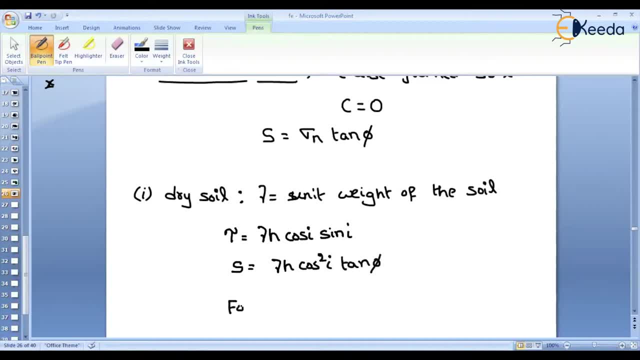 the same. Now find out the factor of safety. Factor of safety will be equal to tan phi S divided by shear strength. divided by shear stress, that will be equal to gamma h cos of square i, tan phi, divided by gamma h cos i sin i. If you simplify this equation, you: 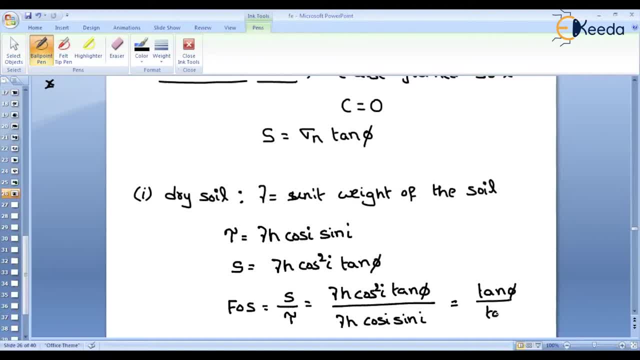 will get tan phi divided by tan i. So if your soil is in dry condition, then the factor of safety of an infinite slope will be nothing but a tan phi divided by tan i. That means, by comparing the angle of friction and the slope of the soil, we can say whether the soil 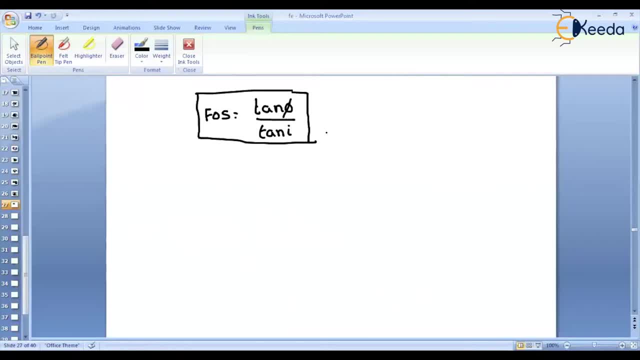 will be in a stable or it will be unstable condition. So this is with respect to if your soil is in dry condition. In the next case, let us say if your soil is in a stable condition, if you are talking about your slope is under submerged condition. 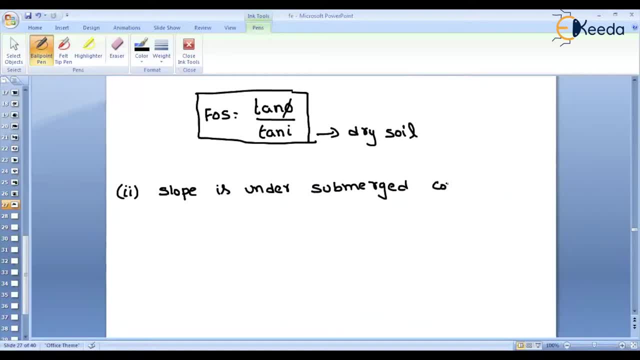 Submerged means what? Your complete slope is under water. So if it is under submerged means there is no flow of water along the slope. This point you have to understand. Okay, Suppose if I say If my slope is under submerged condition, then it is completely filled with the water. 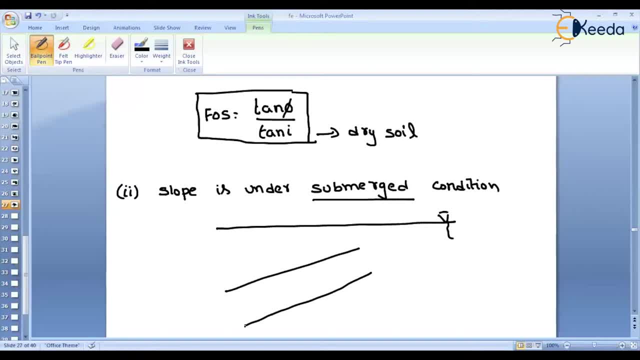 If it is completely filled with the water, then, wherever the point you are finding, the factor of safety, as the soil is completely submerged. As the soil is completely submerged, then instead of taking the unit weight of the soil, here we have to consider the submerged unit weight, while calculation part we have to 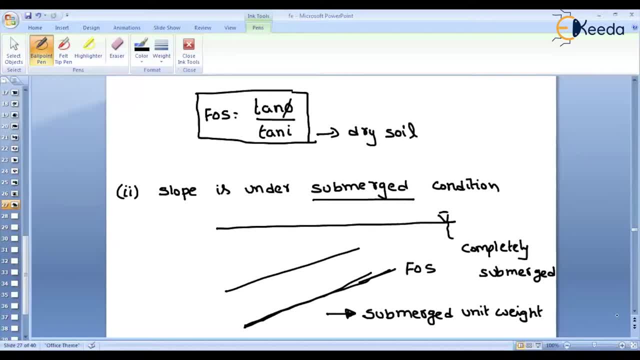 consider submerged unit weight. So if you do the similar procedure for finding the factor of safety, again the same thing. factor of safety will be equal to shear strength divided by shear stress acting on the layer. Shear stress will be equal to if it is a cohesion. 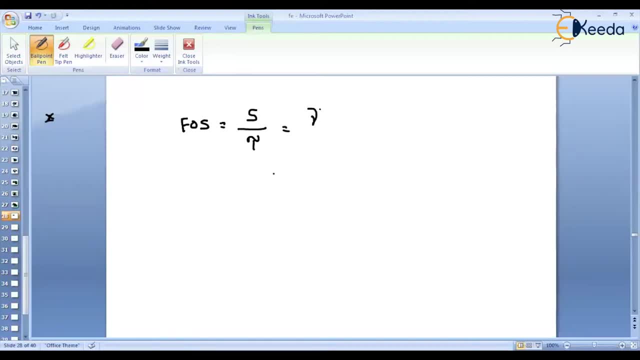 less Sigma and tan phi. Sigma and tan phi is nothing but a. instead of using unit weight, it will be equal to the shear strength acting on the layer. So if you find that the factor unit weight of the soil- here i will use the submerged unit weight gamma- dash into h, into 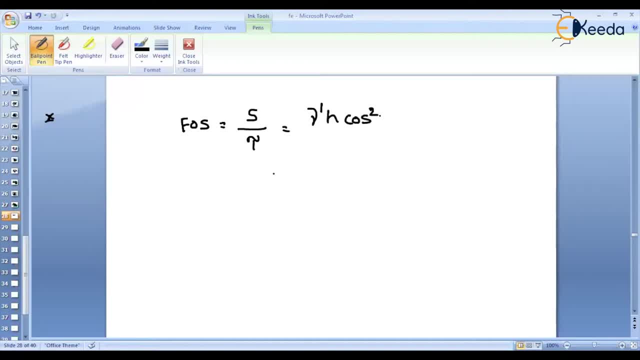 cos square i. tan phi divided by shear stress is nothing but a gamma. dash h into cos i, into sine i. so if we simplify this equation again, the factor of safety will be equal to you will get tan phi divided by tan i. so this is the factor of safety of an infinite slope. 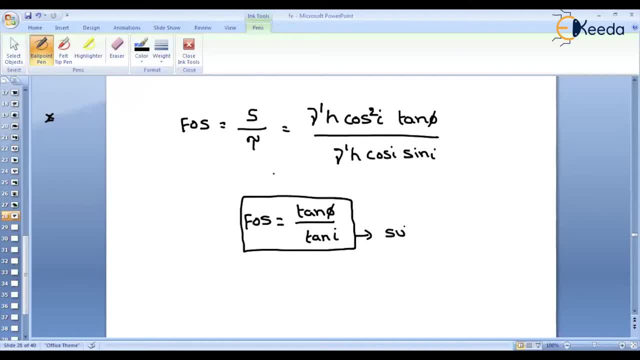 if your slope is under submerged condition. that means whether your slope is completely dry soil or whether the slope is completely submerged. so wherever you want to find out the stability of the slope, you will get tan phi divided by tan i. so this is the factor of safety of an infinite slope. 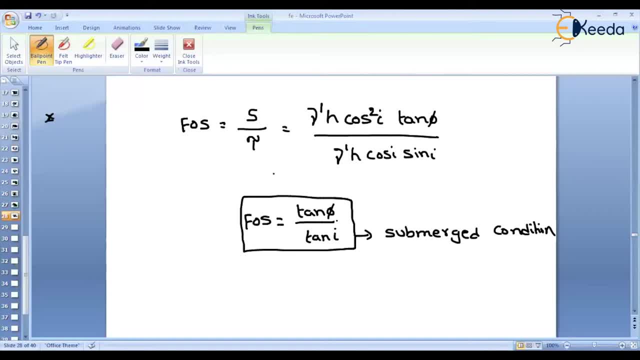 then the simple is nothing but a tan phi divided by tan. i phi is nothing but an angle of friction and i is nothing but a slope of soil, slope with respect to horizontal. in the next case we will discuss with slope, with seepage conditions. let us discuss the third case, that is. 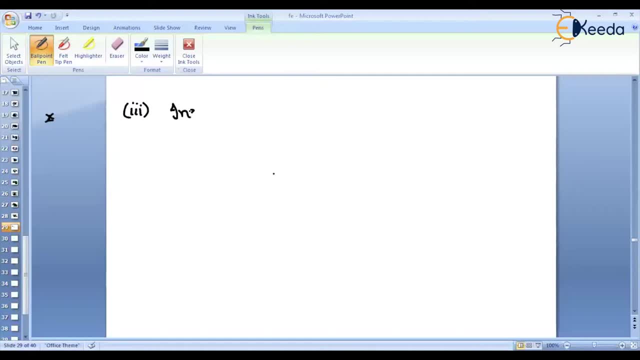 infinite, cohesionless, infinite cohesionless slope with see, the important term is nothing but a seepage. if i am saying you that your slope, your slope is with, seepage means nothing but a. your slope is not completely under the water. what happens is that if rain is happens and 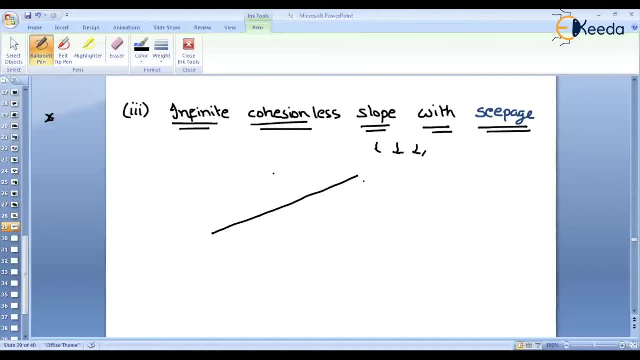 what will happen. whatever the rain happens, then the rainy water will flow through the soil, so this is called the seepage condition. let us say you have infinite slope and let us assume that you are finding the factor of safety at an height h from the ground surface and on the infinite slope there is a seepage condition. 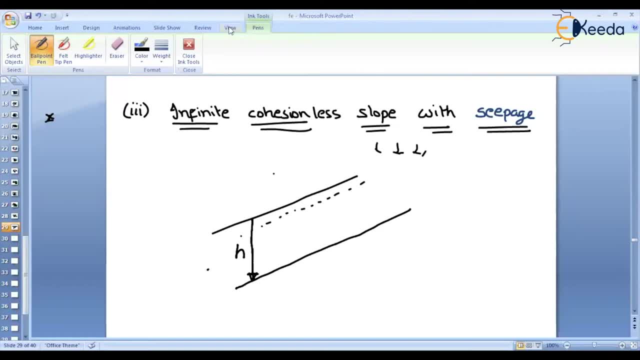 and seepage occurs at a distance of. seepage occurs on the infinite slope at a height z from the failure plane. that means if you are finding the stability along this failure plane, then your seepage is occurring up to a height of z from the failure plane. 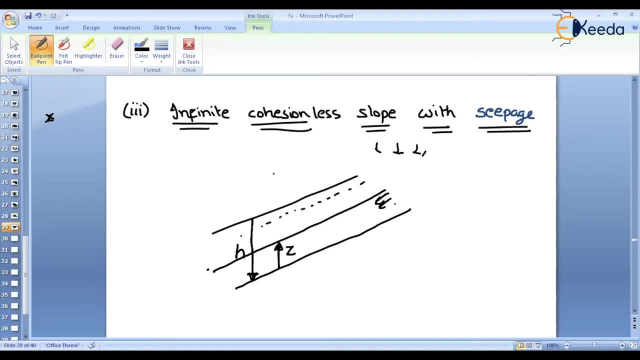 let us say, up to this height the water is flowing through the soil. so understand the difference. that is occurs situation not disturbed. coordinating flow distance between the two sides. therefore, red for that vector, table 빠. So understand the difference. This is not comes under the submerged condition. In the submerged condition, water flow will not be there. Water flow will be only there if you are having only seepage condition. That means the water will flow from higher level to the lower levels. 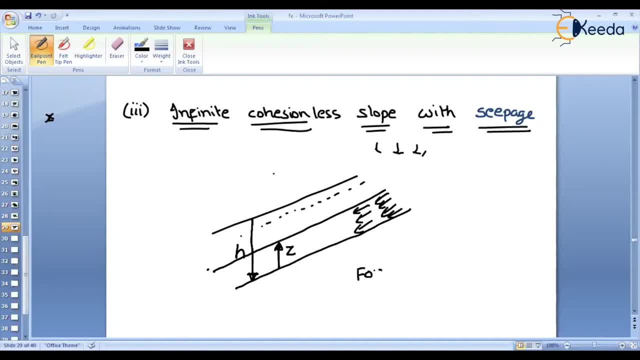 In that case the factor of safety is nothing but a 1 minus gamma w into z divided by gamma, into h, into tan phi divided by tan i. So this formula, we have to by heart it for the gate exam. Okay, this formula we should not derive it in the gate exam. If there is a seepage condition, we should not derive it in the gate exam. 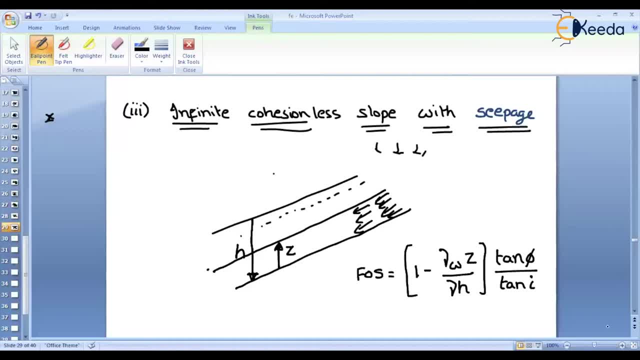 By using this formula we can directly find out the solution. So once again, let us explain the terms under it. So again I am rewriting the terms: Factor of safety equal to 1 minus gamma w into z divided by gamma into h times the tan phi divided by tan i. 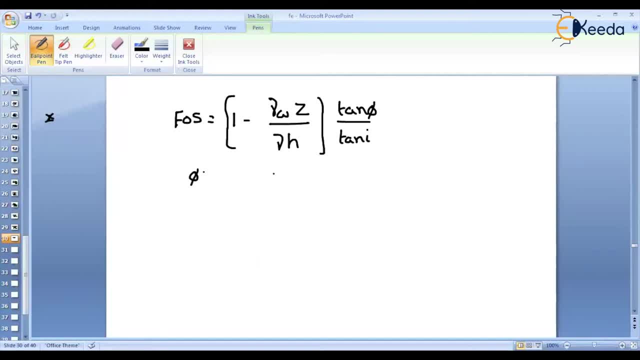 Already, we have seen some of the terms. What are they Here? phi is nothing but a 1. Angle of friction, i is nothing but a slope and h is nothing but a distance to the failure plane. Distance to the failure plane. 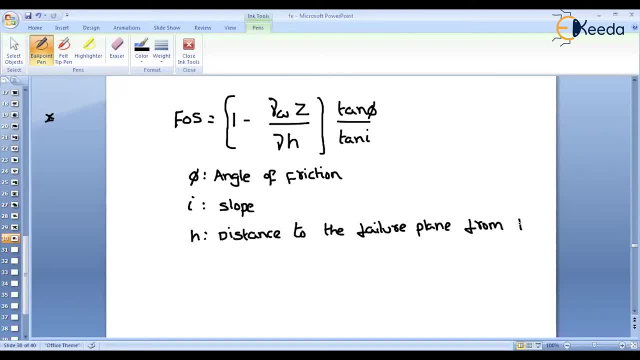 From the ground surface and z is nothing but a distance from failure plane to the seepage level. Okay, and the gamma w? it is nothing but a unit weight of the water and the only the remaining term is nothing but a gamma. Gamma is nothing but a average weight density of the soil. 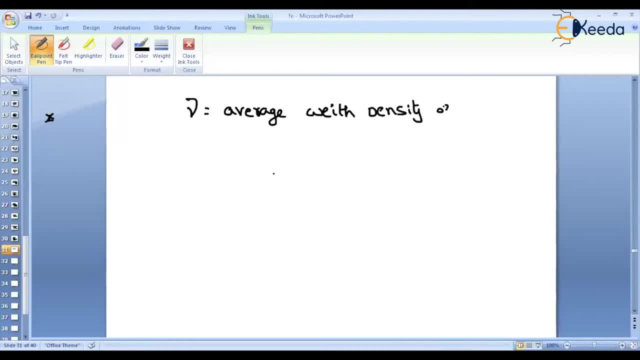 Average weight density of the soil. Okay, that means let us consider Again. I am rewriting the diagram. Let us assume this is where we are finding the stability. That's why I am calling it as a failure plane. My failure plane is at a distance of h from the ground surface, and also there will be a seepage in the infinite slope. 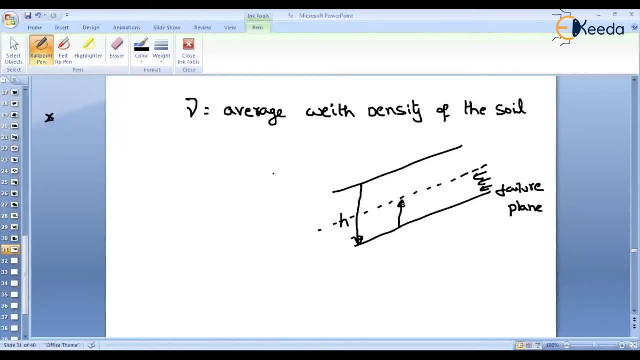 So the distance between the failure plane to the seepage flow, that is nothing but a z. So from here to here the soil is in the dry condition. Let us assume that In this level the unit weight, that is nothing but a, let us say gamma. 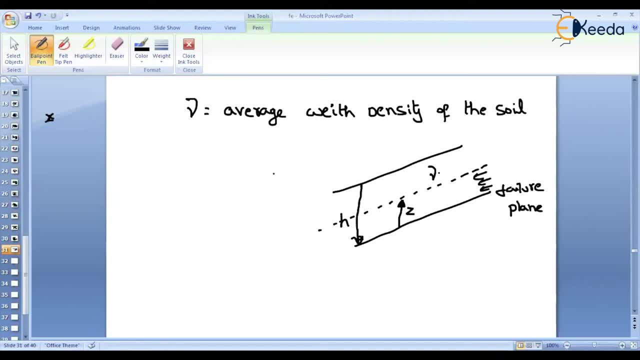 Let us replace this with, okay, gamma dash. So the gamma dash is nothing but a submerged condition. Let us say I am representing this with the gamma subscript 1.. From here to here, the soil is under this saturated condition. 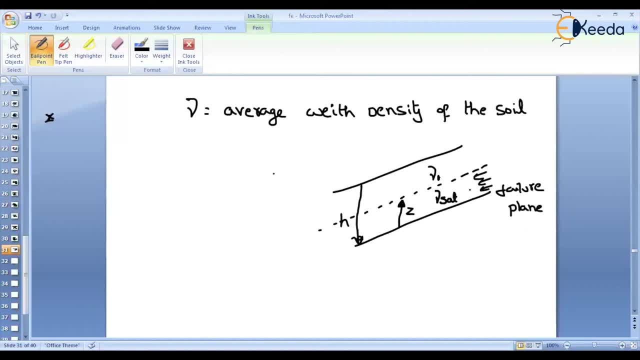 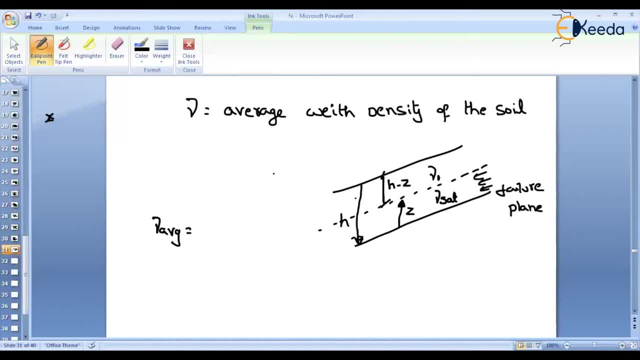 h minus z. So what is the total weight in this span? Gamma 1 into h minus z plus from here to here. gamma set: Gamma set into z divided by h minus z plus z, So z z gets cancelled. 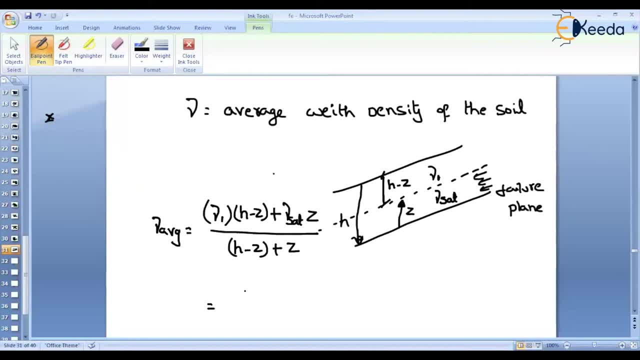 Then you will get divided by h, So that will be equal to gamma 1 into h minus z, plus gamma set into z divided by h. This is what we will use: the gamma average. By using this equation we can find out the factor of safety if there is a seepage flow. 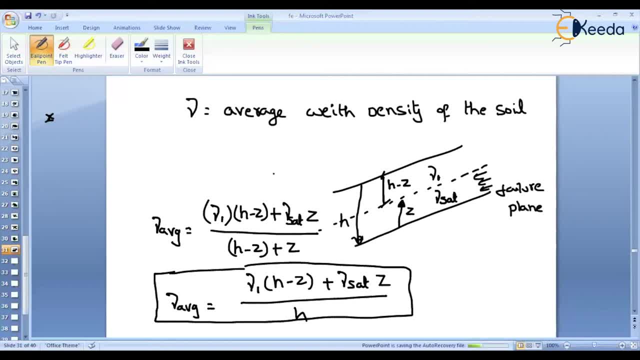 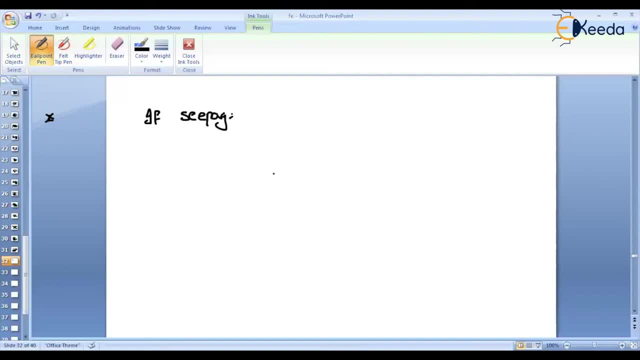 Let us consider a case that if seepage level passes through the ground surface, passes through the ground surface, or also we can call it as a ground level. That means consider an infinite slope Here. it is not under submerged condition. 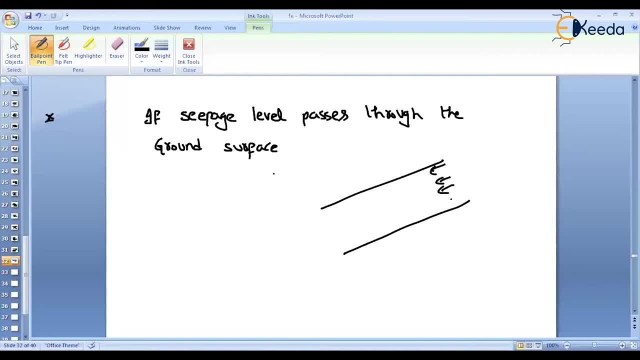 The seepage flow, the seepage flow that is acting from ground level to the failure plane. So, in this case, what is happening? If this is your failure plane, so this is nothing but a h, So as the seepage flow is up to the ground surface, 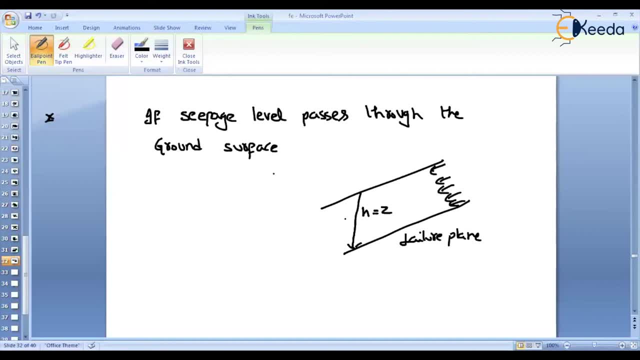 then we can say h is equal to z. So in this case, what about your average weight density? Your average weight density is becoming the as complete soil is. under the saturated condition, that will become the gamma z. I can recall the equation: factor of safety. 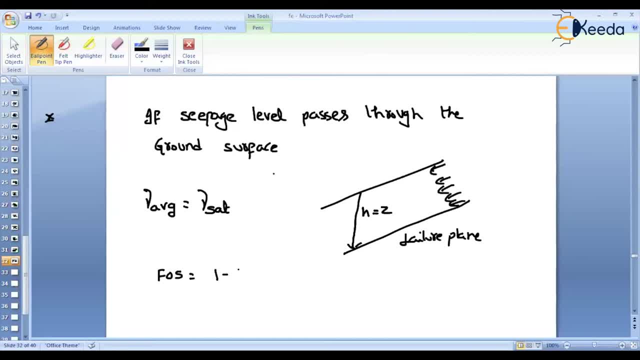 If I recall the factor of safety equation, that will be equal to 1 minus gamma w, divided by gamma average into h, divided by sorry z, divided by h, z divided by h into tan phi, divided by tan i, z and h gets cancelled as the seepages occur up to the ground surface. 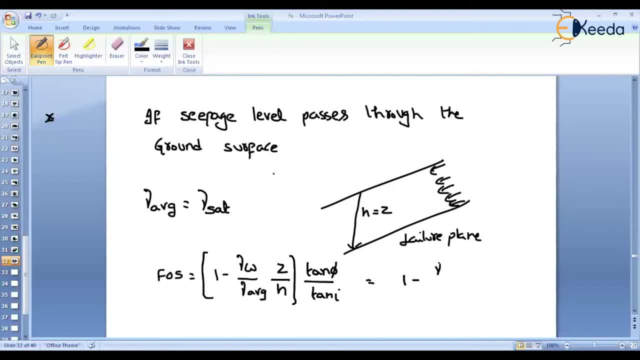 So if I simplify this equation, how I will get 1 minus gamma w divided by gamma average, into tan phi divided by tan i? So sorry, this gamma average is becoming nothing but a gamma saturation. So, instead of the gamma average, what I will write, 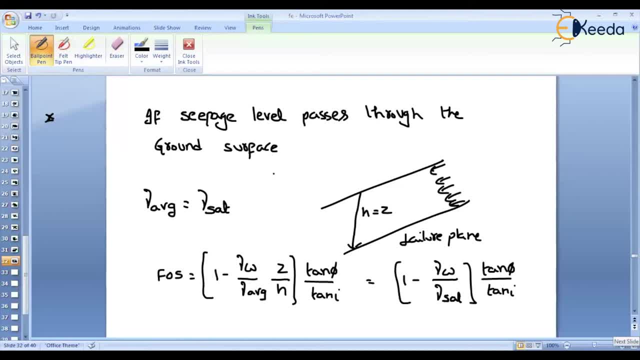 I will write it down as a gamma saturation For soils. we can say the gamma saturation, or else we can say the weight density of water that will be become as half of the gamma saturation. This is not exactly equal to. we can say approximately equal to. 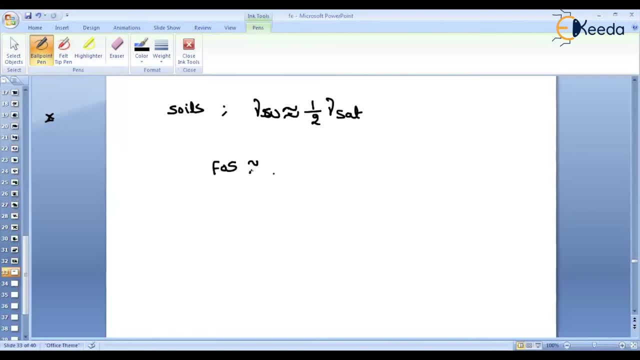 So that's why what I will say, my factor of safety is approximately equal to 1 minus instead of gamma w. I will write it down as: 1 by 2 gamma saturation. 1 by 2 gamma saturation. 1 by 2 gamma saturation divided by gamma saturation into tan phi divided by tan i. 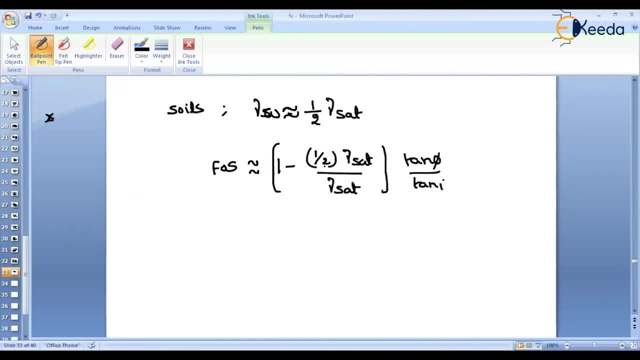 So gamma saturation, and gamma saturation gets cancelled. 1 minus 1 by 2 is nothing but 1 by 2.. So, factor of safety, it is nothing but a nearly tan phi, 1 by 2 times tan phi divided by tan i. 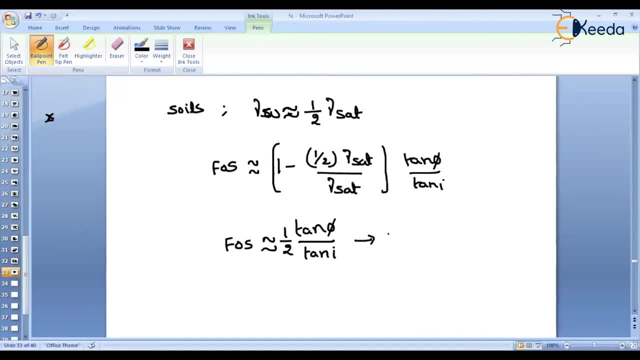 This is the factor of safety when your slope is under steady sea page up to ground surface. So every time this equation may not be possible, but if they are asking you about the specific value, we have to substitute the gamma set value.